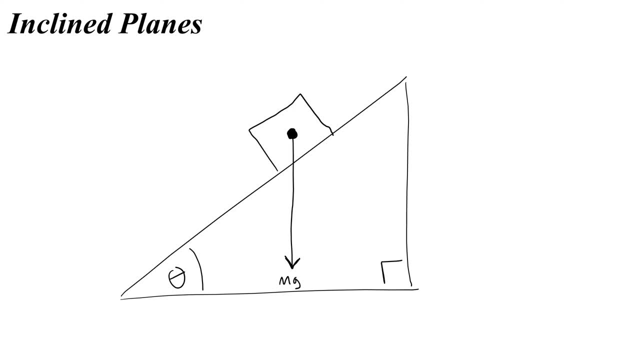 A, dA, mg. Okay, good, What about the normal force? The normal force is still going to be perpendicular to the surface, which means it's going to look like this: Incredibly annoying. This makes problems kind of difficult because the normal force and the weight are no longer in the same. 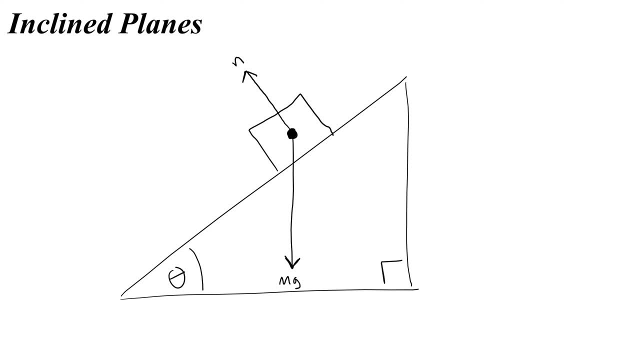 uh line right, they're no longer both y forces, um, and we could do a couple of things. first of all, we could take the normal force and try and make an ny and nx. that's totally fine, sometimes people do that, but what i think is a lot easier to do is to take the weight and to learn how to take. 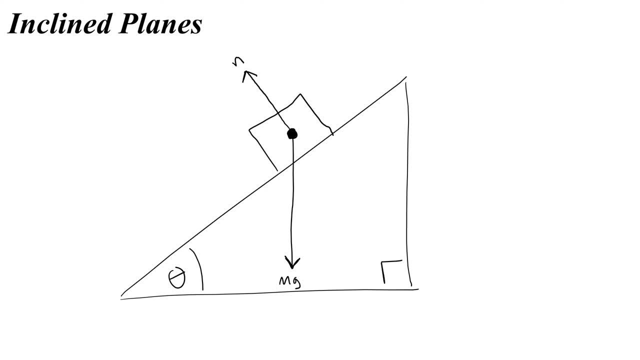 turn the weight force into an x and a y component, but instead of x and y it's parallel to the ramp and perpendicular to the ramp, so like a parallel and a perpendicular axis. so let's do that for the weight force. what that looks like is i'm going to make a right triangle that looks like this: 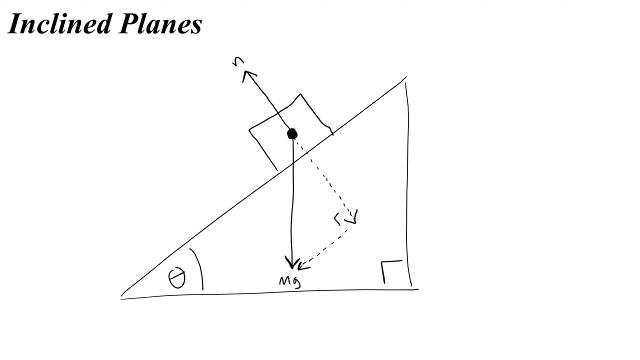 okay, so that's the right triangle. okay, so if i do this, um, i can think of out how much of the weight is pushing into the surface, and therefore what the normal force is, and then how much of the weight is going down the ramp, which is important because only a certain 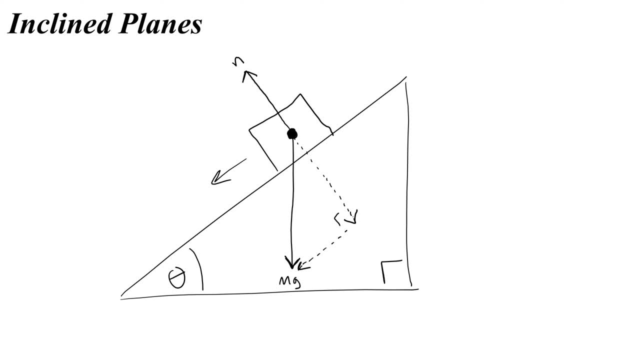 portion of the weight force is going to be down the ramp and cause the box to accelerate, or anything like that. so, but how much? how do i figure it out? well, to do this, i have to decide: does my angle of inclination. theta belong here or here? well, the key is that we always put the angles. 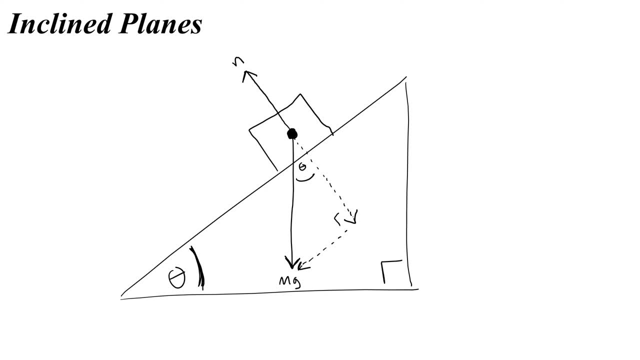 at the tail end. so it's going to be here, but let's talk about the geometry of that real quick. basically, if i draw a line parallel to the ground and then i draw a line that's perpendicular- sorry, perpendicular- to the surface, then i'm going to notice the whole like alternating. 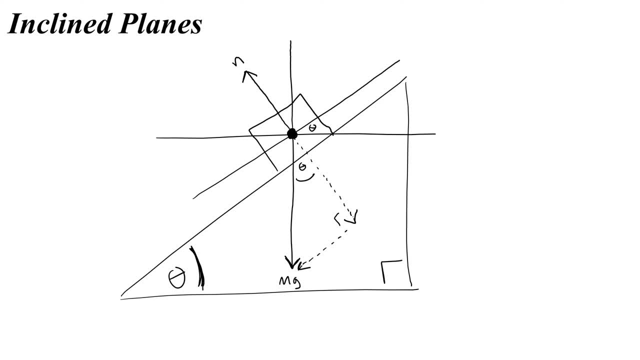 interior angles thing, where this would be theta and this would be some other angle, i don't know. we'll call it beta, and then this would be beta and this would be theta, theta and this would be beta, and this would be theta and this would be beta. you know what i mean. 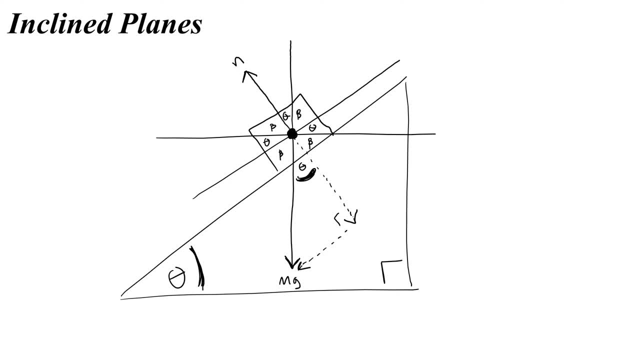 so theta is what goes here. but if you don't like geometry, you can just sort of memorize this fact that we always put the angle by the tail right here. now. the other thing that we can do is is think about what part of the weight- cosine or sine- goes where. so this component right here. 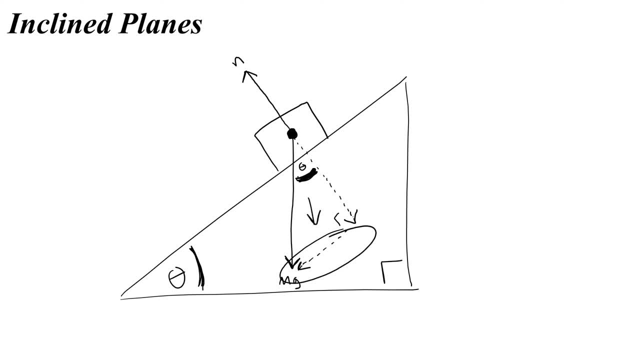 it points down the ramp and it is opposite of theta. so we would use sine for this component. it would be mg sine theta. and then we would have this component here which is adjacent to the angle, so it would be mg cosine theta. now the way that i like to think about this is: mg sine theta goes down the ramp and i think, like some, 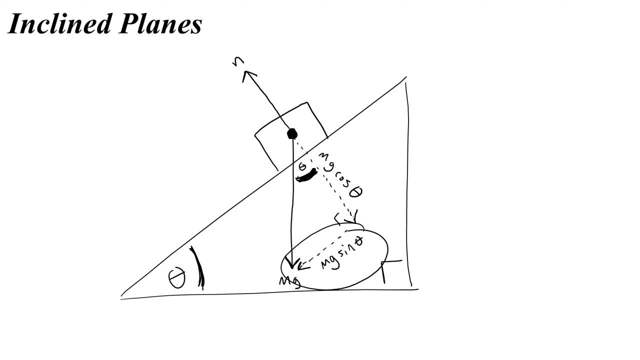 annoying fact, little reminder to myself: it's a sin to go down the ramp like you're like a. you're like a bad kid and you're not supposed to get on the ramp or the slide because your parents will get mad at you and you have been taught that it's a sin to go down the slide and so sign always: goes down the. 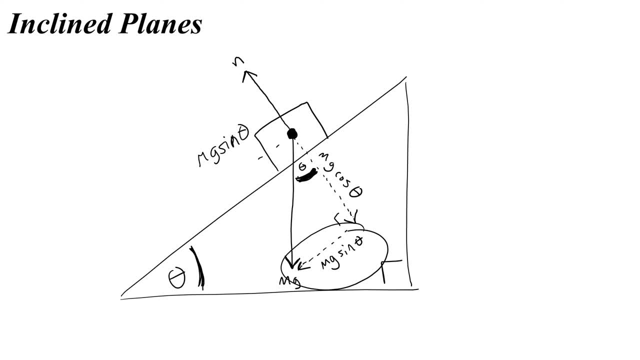 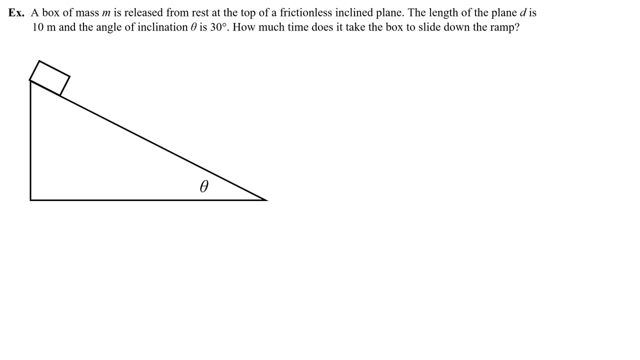 inclined plane. it's totally stupid, but it works. so sign goes down the ramp. it doesn't go down the ramp. you don't want to be one of those, those nasty skateboarders who are doing evil skateboarding? no, okay, anyway. so here's how we use these components in problems. oh, you know what? and first i should. 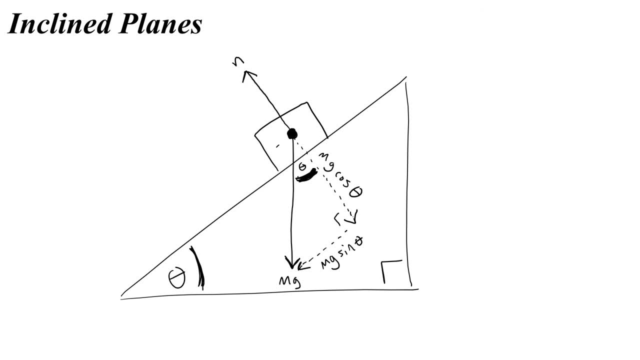 say this. so basically, in this very simple example, with no friction, we would say that the mg cosine component is equal to the normal force, mg cosine theta- really important- and this mg sine theta thing. this is an unbalanced force, so it would be equal to the mass of the box times the 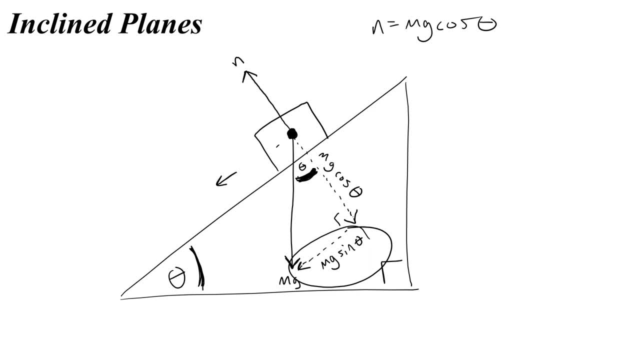 unbalanced force, so it would be equal to the mass of the box times the unbalanced force acceleration. now, if you can imagine, when this box accelerates, it's going to accelerate parallel to the ramp and this mg sine theta is parallel to the ramp. so what i can do is i can say mg sine theta. 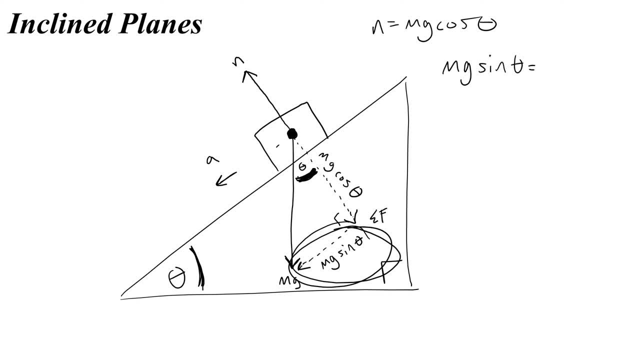 is equal to mass times acceleration, because it is the net force. and when i do that, you'll notice that the mass cancels out and i found that the acceleration is g times sine theta. if i can, if there aren't, if there isn't any friction, if i can ignore friction from the ramp. 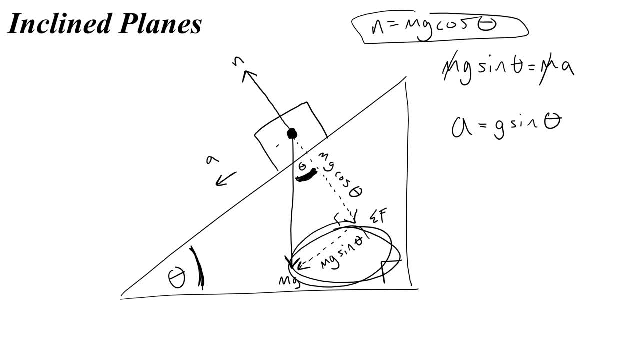 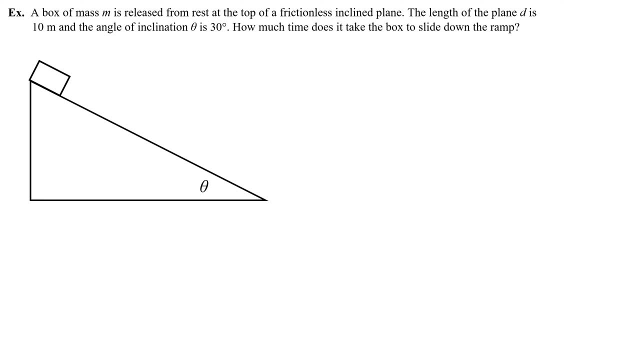 okay. so if there was friction, i would use that for the normal force, and then, of course, i would have to change this equation. so let's see what this looks like. a box of mass m is released from rest at the top of a frictionless inclined plane. the length of the plane is d. our plane d is 10. 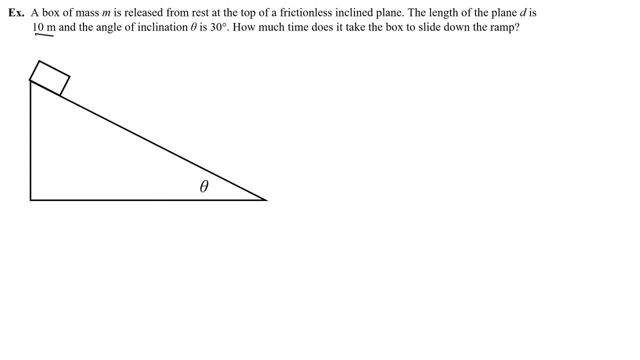 meters and the angle and inclination theta is 30 degrees. how much time does it take the box to slide down the ramp? so i'm going to use this equation and i'm going to use this equation and i'm going to scale thisliciton, ordering it everywhere on the ramp. okay, so a couple of things released from rest. so the initial velocity is zero. 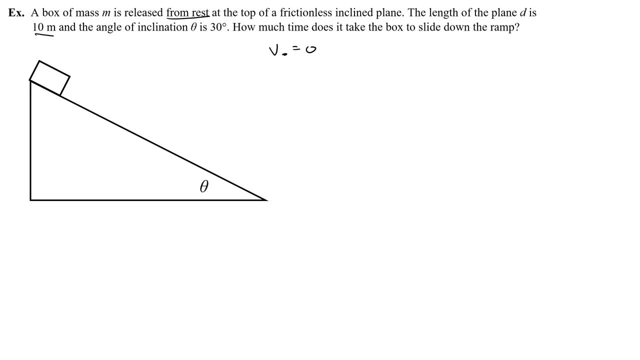 um, the distance that it travels. d is 10 meters. so what i could do is i could think like um. it's like saying that your x naught is 0 and then the final x that you reach is 10. right, we're sort of saying like delta, x is the distance d. 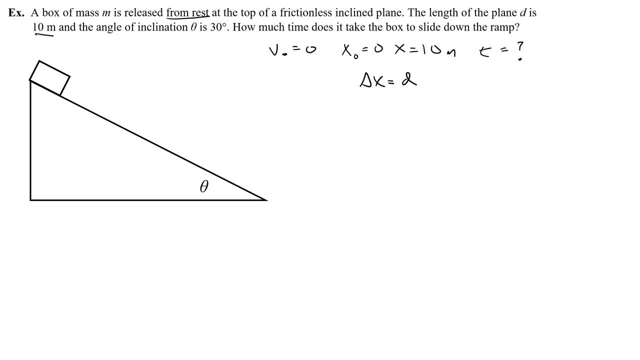 um, and also, oh, you were asked to find t, so how do you do that? well, i'm going to. he is this, this half, in all the ways i've put in the? Well, I'm going to use a motion equation that has an acceleration in it, right, 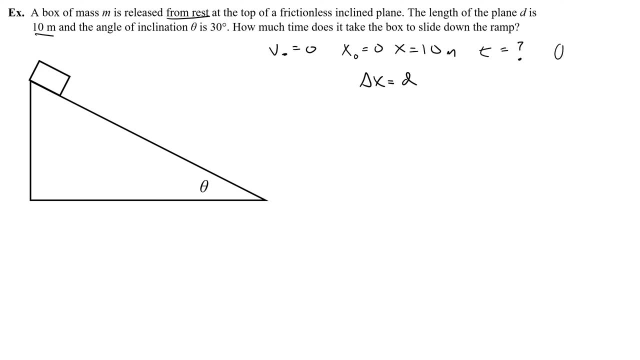 Because this is a problem where I can look at force and I know that acceleration is always equal to net force divided by mass. So if I can figure out what the acceleration is, I can maybe use it in a motion equation to solve this problem. 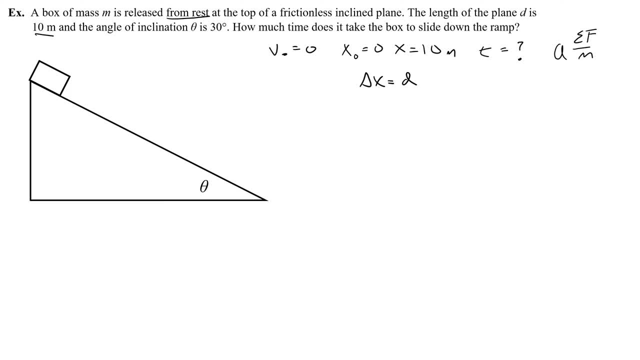 Now, before we get into the forces, let's talk about the motion equation. that would solve this problem. I have the initial velocity stuff about positions and time, So the equation for that is going to be: x equals 1, half a t squared plus v naught. t plus x naught. 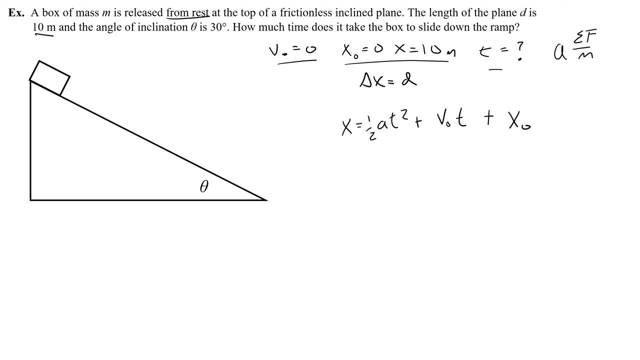 And basically what I'm doing is I'm saying that delta x is d and it's 10 meters, So I'll just write this as delta x And instead of delta x I'll call this d. The initial velocity is zero, so I'll get rid of that whole term. 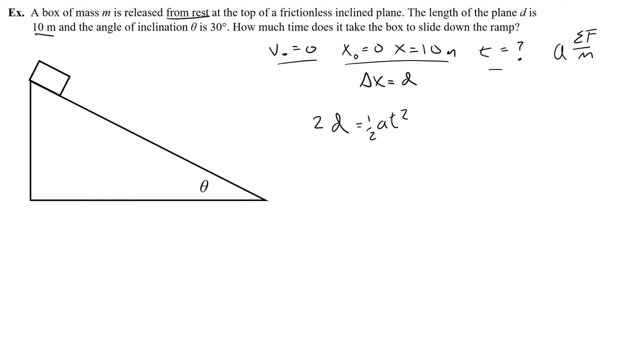 And here we have our equation: Define time, Multiply- I have- both sides- by 2 to get rid of the 1 half, Then divide by the acceleration And ultimately take the square root Right. so I'll save this equation. 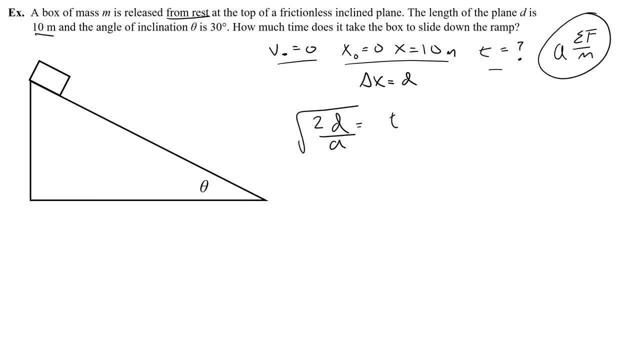 I've already worked it out. Once I know what the acceleration is, by taking the net force divided by mass, I'm going to take the square root of 2 times 10 over the acceleration. Okay, so put that onto the side and let's talk about how can I find the acceleration. 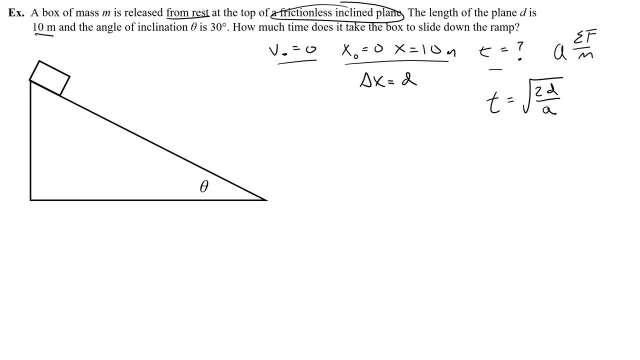 Well, it's a frictionless inclined plane. So this problem is going to have a weight force down- mg- and a normal force up. And this is where we do the parallel and perpendicular components thing. I draw the perpendicular component and it's mg, cosine, theta- and the parallel which is 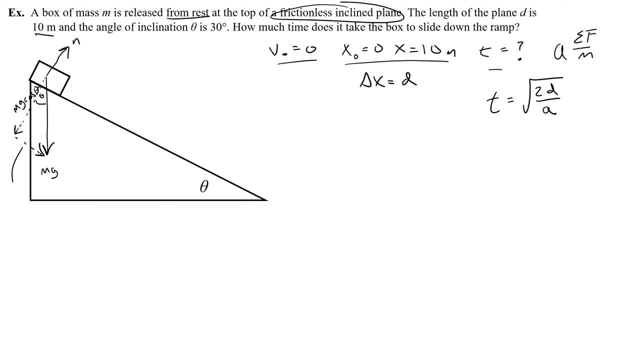 the part that goes down the ram, mg cosine theta, m g sine theta, And I don't really have to draw the geometry for this, I can just remember it's sin to go down the ramp. Now sometimes, remember you can draw components wherever you want. 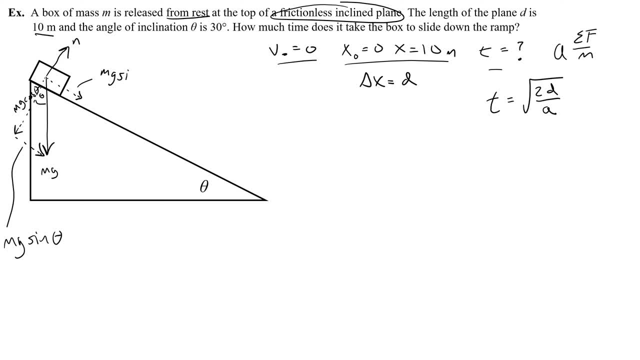 but it's easier to think of this m g sine theta kind of coming out like if we move that component up, because that helps you understand the part of the weight that's going down the ramp and causing the box to accelerate. Okay, so in this problem, what do I need? I need m g sine theta because it's 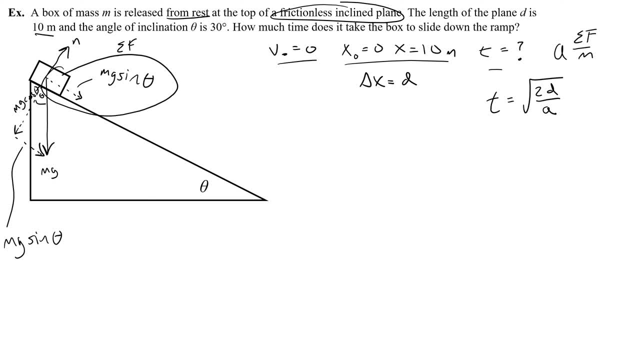 the unbalanced force And, just like we were talking about before, it will be equal to the mass times acceleration. I don't care about the mass, it goes away. and I've just proved what I showed before: Without friction, the acceleration down an inclined plane is g times sine theta. 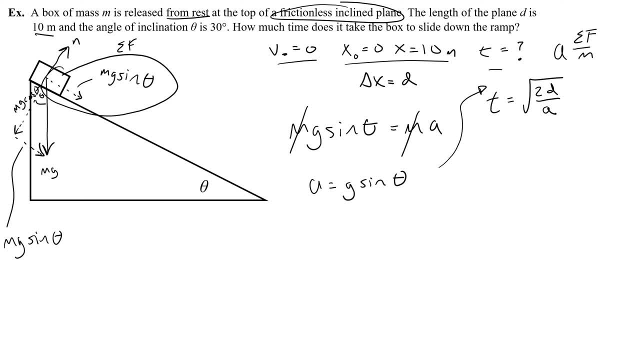 So that is what I can put in my equation here. If I want the time, take the square root of 2 times d over g, sine theta, So the square root of 2 times 10 meters over 10, we'll use that for g meters per. 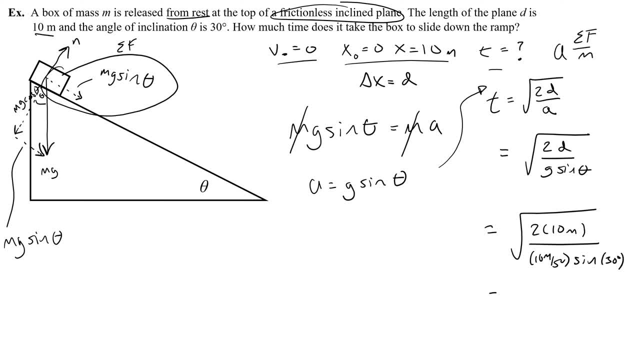 second squared times, sine of 30 degrees, And if you knew what sine and cosine of 30 was, then you could perhaps get a fraction for that. Of course, sine 30 is the easy one, right, It's one half. 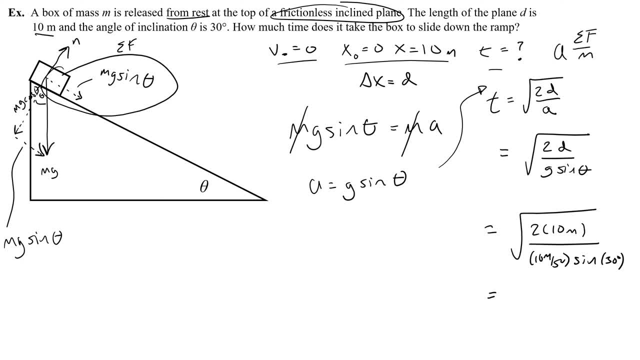 and half of 10 is 5, and then 2 times 10 is 20,, so 20 over 5 is 4, and the square root of 4 is: did you get it? 2. Takes two seconds to go down the ramp. Okay, let's do a problem. that is a little bit different. 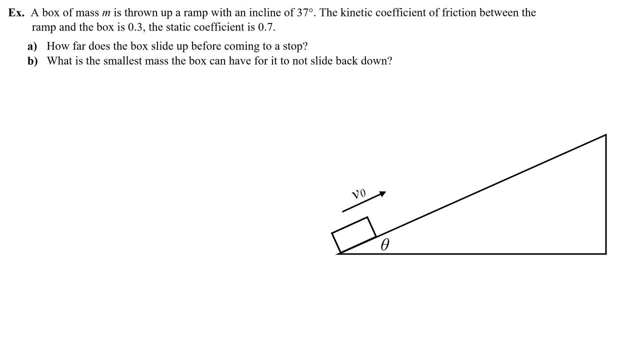 A box of mass m is thrown up a ramp with an incline of 37 degrees. The kinetic coefficient of friction between the box and the ramp is 0.3, the static coefficient of friction is 0.7.. Okay so, before we, 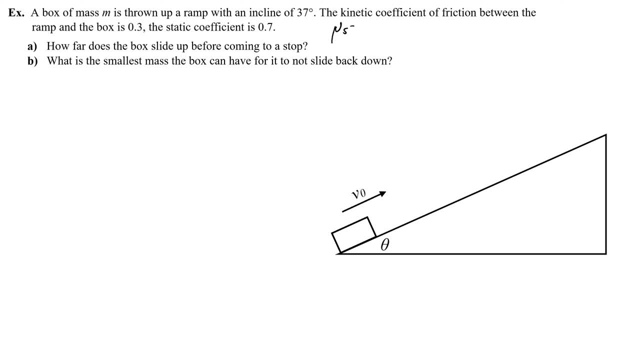 get into A and B. let's write down that information. They told me mu s is 0.7,, mu k is 0.3, and an incline of 37 degrees, so theta is 37. They didn't tell me what the mass is. 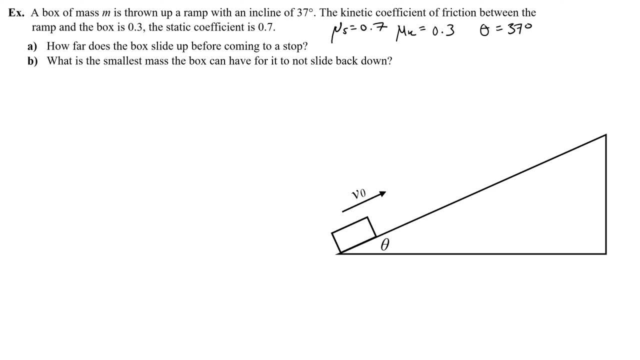 so that's a clue that I might have to cancel it out. Hint, hint, Okay and A. how far does the box slide up before coming to a stop? Oh yeah, the initial velocity- You know, I think this is supposed to say v-naught- equals 10 meters per second squared, Sorry. 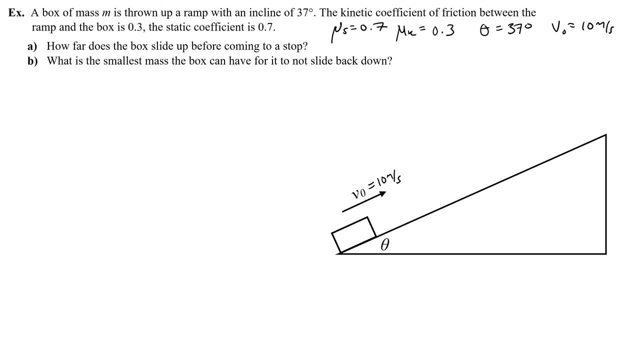 Should have said that in the problem. Okay so, initial velocity: 10 meters per second. Great. So how far does the box slide up before coming to a stop? Well, what does that mean? That means that this box is going to go up the ramp and eventually get to this place where it has a velocity of 0. 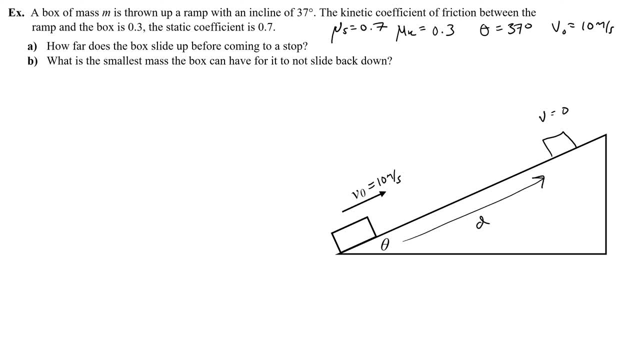 And what we're trying to do is figure out what is that distance? Now notice that I'm using d-naught x or y, because technically there's like an x-naught- y-naught coordinate and then an x comma y at the end, and that's just dumb. 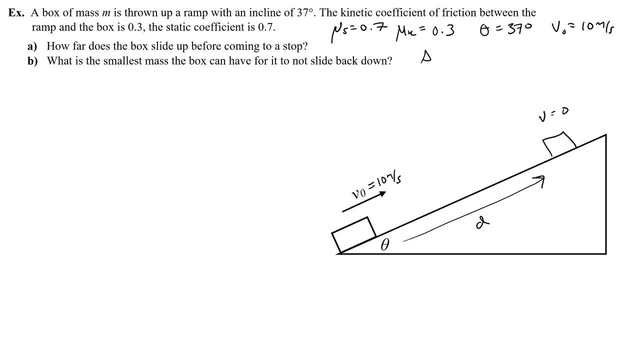 So we're just thinking of it in raw terms of the distance. Delta x in our equations is just the distance and it's what we're looking for Now in this problem. you're given the initial velocity, You know the final is 0, and you want to find d. 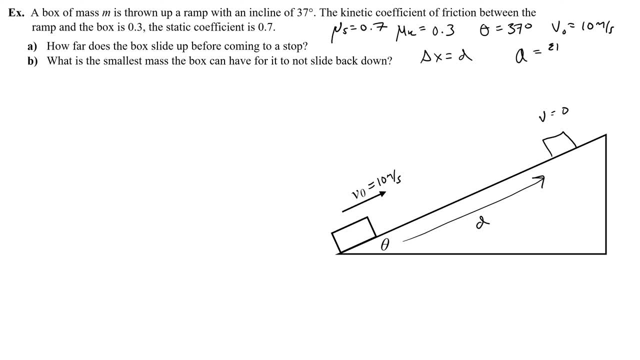 and you know that you can find the acceleration by taking the net force, if you can figure it out, and dividing it by the mass. So the one thing that you don't have or are told about in this problem is time. So that's a hint that to solve part a you're going to use the ain't got no time equation. 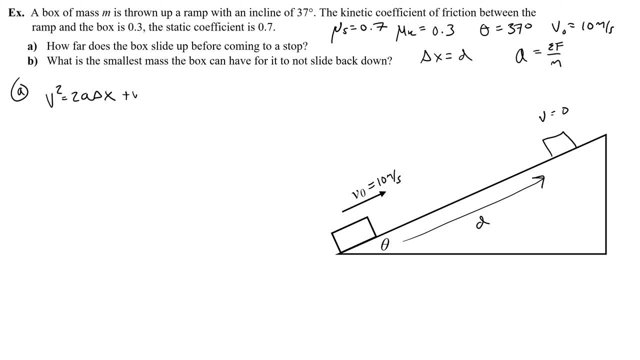 v squared equals 2a delta x plus v-naught squared, where instead of saying delta x, we're just going to call it d, so 2a d, and the final velocity is 0, so we're going to get rid of it. 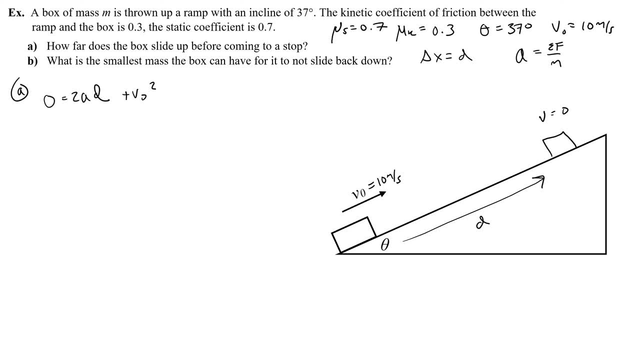 Okay, so in this problem you want to find d. I'll just go ahead and organize the equation so that I'm ready to solve it. Subtract v-naught squared from both sides, Then we're solving for d. so divide by 2a. 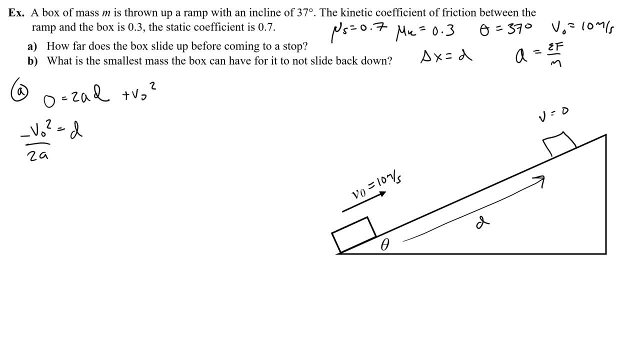 And I can find the distance, what it wants, in part d if I take the initial velocity of 10, square it and then divide by 2 times the acceleration. So let's do that Okay. so now let's talk about the acceleration. 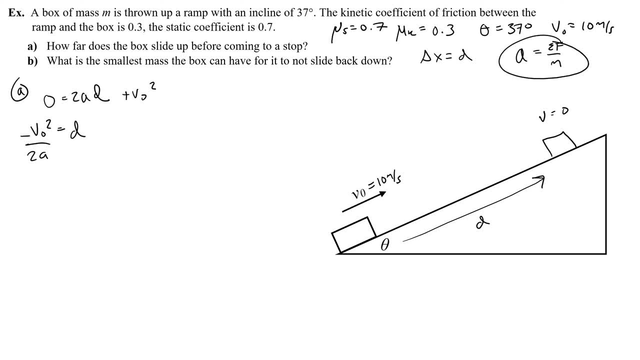 Remember, the clue is that I'm going to be looking at forces, because somehow I'm going to get to a place where a bunch of forces equals mass times, acceleration. So what do we have on this box? Well, as it goes up, the weight points down the entire time and immediately I'm going to draw the normal force perpendicular. 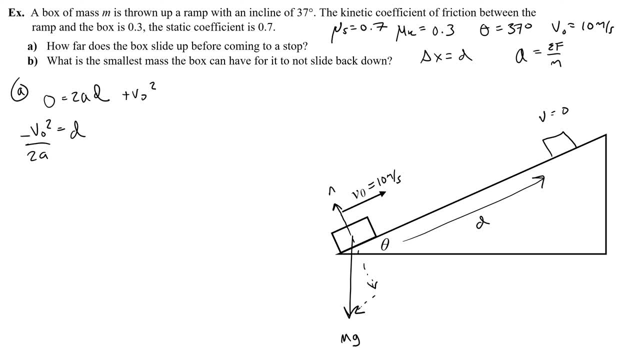 and then my parallel and perpendicular components. It's hard to do sometimes, So I'm going to do a cosine. it's adjacent to theta and then it's a sin to go down the ramp. so mg sine, theta points down the ramp. 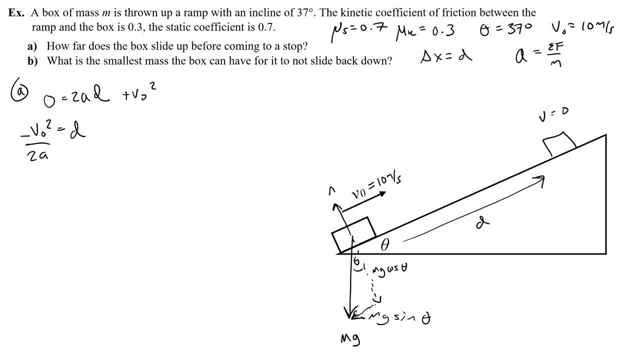 Okay. well, what else is going to be happening to the box as it goes up the ramp? Well, as it goes up the ramp, the force of friction is kinetic because it's sliding up the ramp and will be down the ramp. 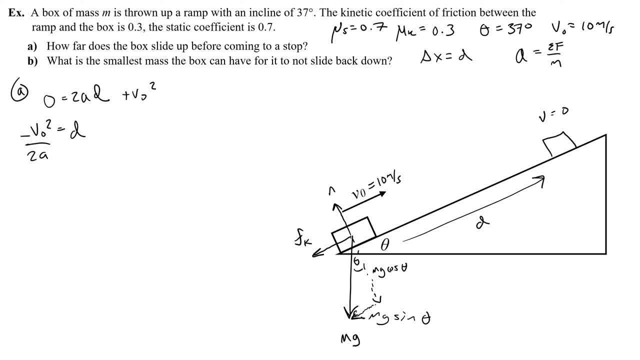 Ooh, wild stuff. Now, at this point I would need to think about whether down the ramp or up the ramp is going to be my positive or my negative, But since mg, sine theta and fk both point down the ramp and that's going to be the direction of the acceleration, 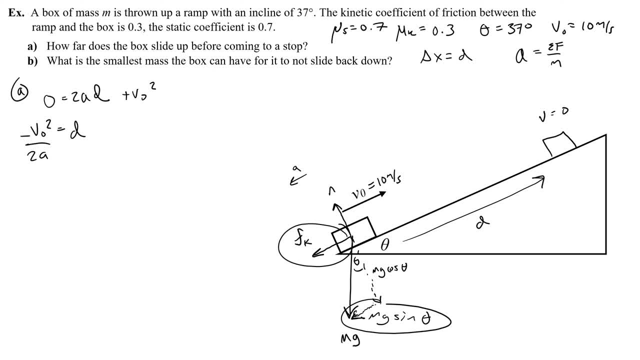 I'm just going to write that as my net force, right? So my net force is mg sine theta plus friction, and then say that that is my net force. so that's equal to mass times. Oops, sorry, Acceleration. So mass times, acceleration. 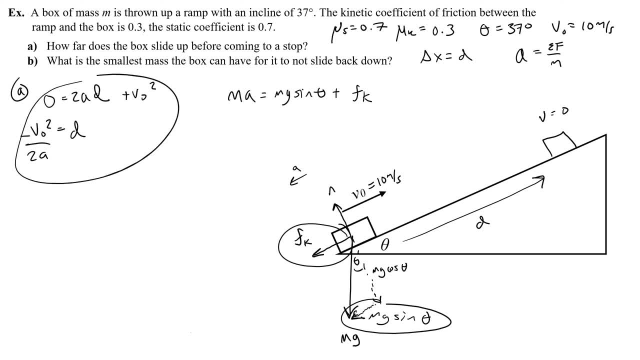 And I'll worry about the motion problem and whether the acceleration be a positive or a negative number. I'll worry about that when I work on the motion part. Okay, So mg sine theta plus friction, they're equal to the net force and therefore mass times acceleration on the box as it goes up the ramp. 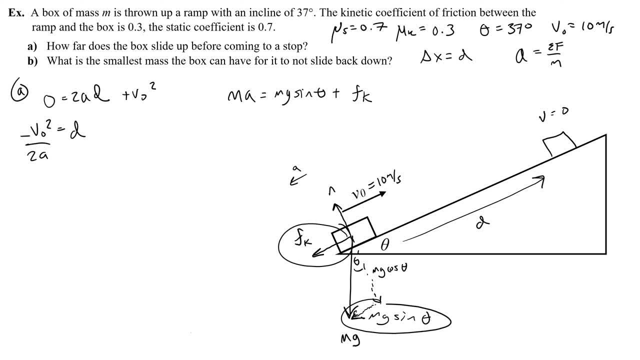 What can I do with this? Well, I have m in most terms And remember I don't know what the mass is. Okay, So what I'm probably going to have to do is somehow get friction with an m in it so that I can hopefully get rid of it. 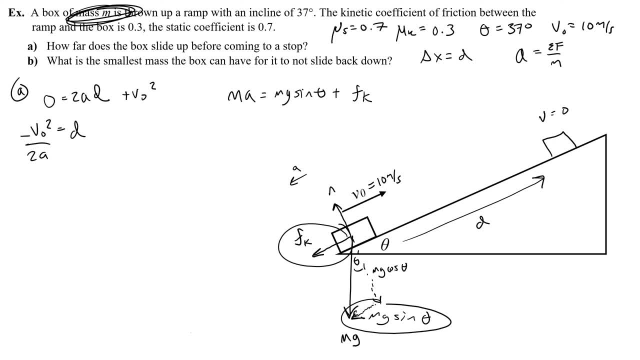 So let's talk about that. What is fk equal to? Well, if I kind of move off to the side here a little dividing line, so we have some space friction is fun. So mu times the normal force, And in this problem the normal force is not equal to mg. 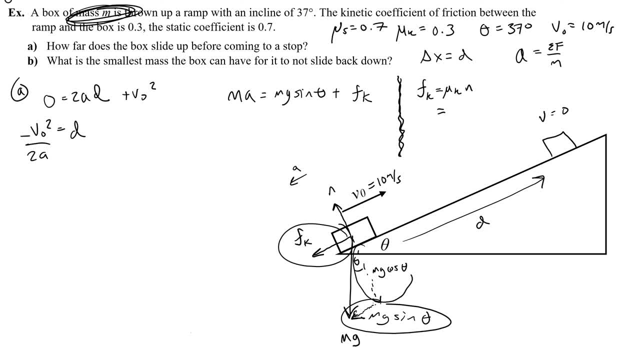 But instead the normal force is equal to. The normal force is equal to mg cosine theta. So we would write mu k mg cosine theta. So that's what I'm actually going to plug in for my equation right here. Let's say: ma equals mg sine theta plus mu, mg cosine theta. 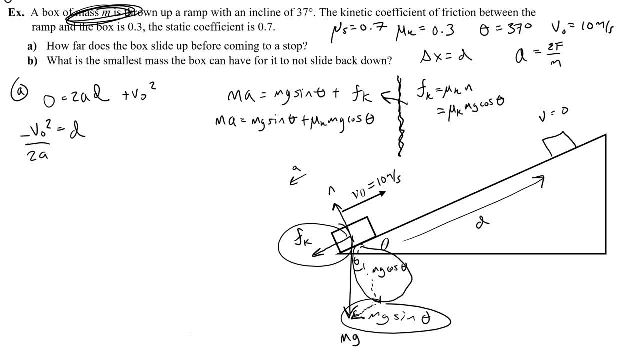 Now, why did I do this? Well, again, there's an m In every term, So now I can get rid of m completely. Yay, And it turns out that I know all of this information, So I can solve for the acceleration. 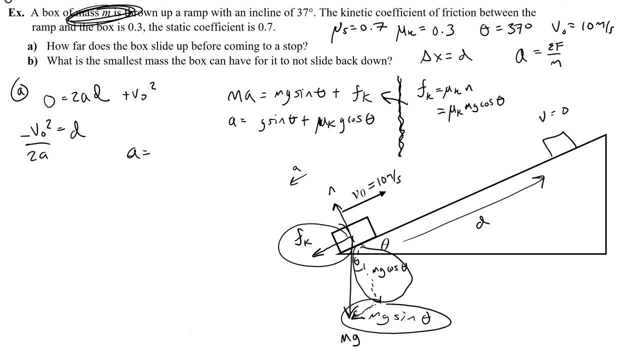 The acceleration is going to be g sine theta, So 10 meters per second squared Times sine of 37.. Cosine of 37 degrees Plus mu is 0.3.. 10 meters per second squared Cosine of 37 degrees. 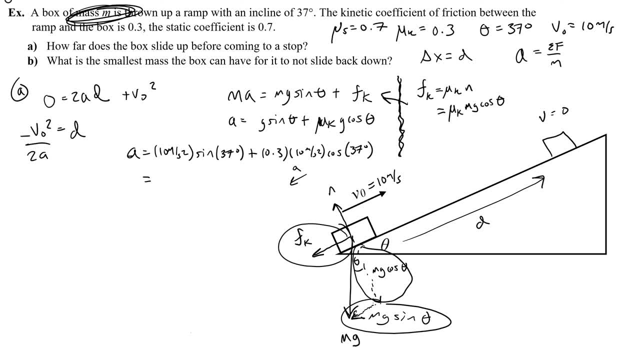 Okay, so that's a big number. I'm going to get 10 sine 37 plus 0.3 times 10 times cosine of 37. That's going to be 8.4 meters per second squared. Okay. so now that I've found the acceleration, I can use that to find my distance d. 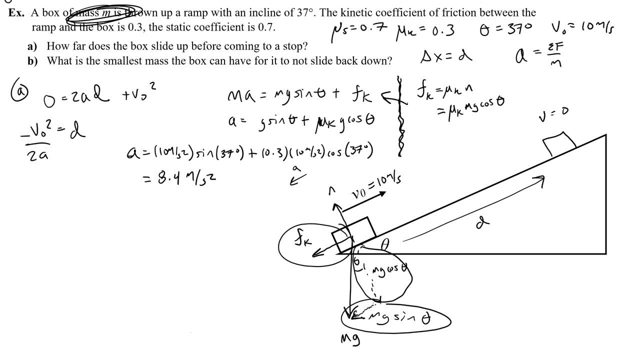 But again, I have to pause here and remember that this acceleration is down the ramp, And so if I want to say that the initial velocity and the distance up the ramp is positive, then when I use this 8.4 in my equation, I need to make it a negative 8.4.. 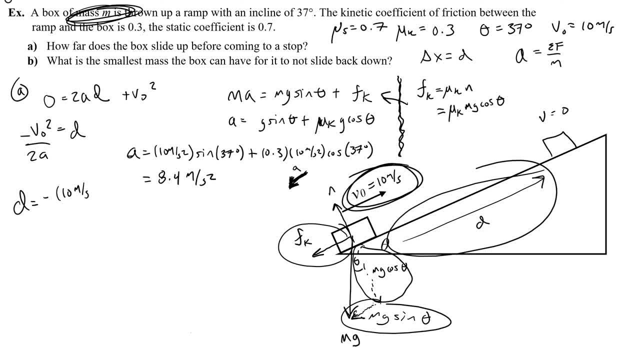 So the distance would be negative: 10 meters per second squared, That's the initial velocity Times 2 times negative: 0.84 meters per second squared. So yeah, I mean when we're thinking about net force and free body diagrams. 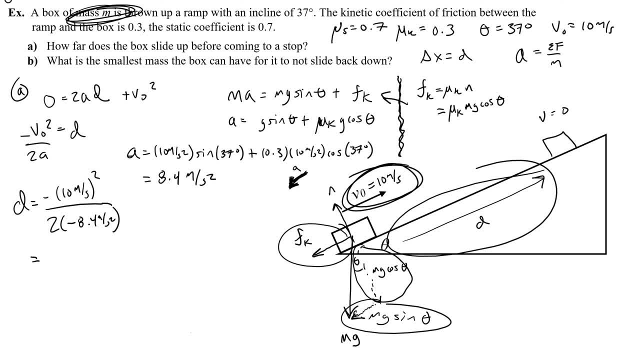 we always want to make the direction of the acceleration positive when we're writing our equations, But sometimes, when we step into like motion world, it would be better for us to make the acceleration negative, which is what we're doing in this problem. 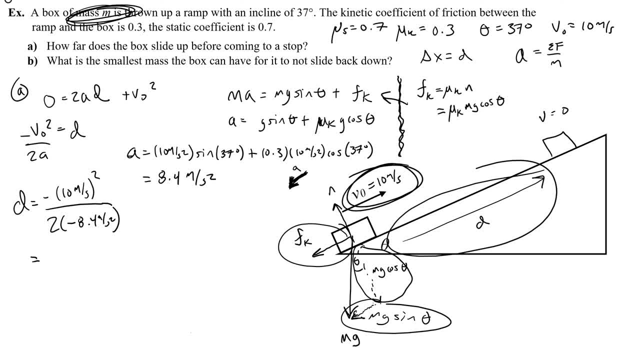 Okay, so negative 100. Negative 100 divided by what negative, like 16.8.. 2 times 0.04.. So that's going to give me a positive 5.95 meters up the ramp. Whew, tough problem. 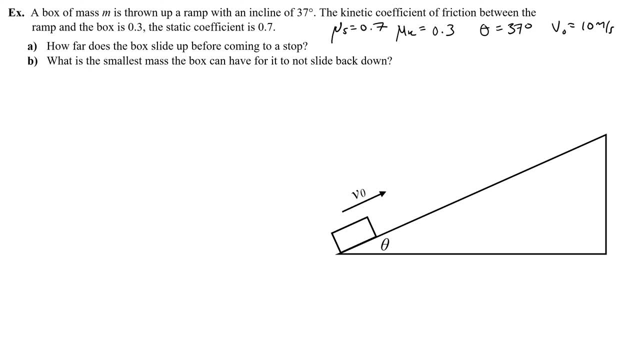 Okay, so now let's talk about part b. What is the smallest mass the box can have for it to not slide back down? Okay, well, so the box is up at the top. It's finally reached a stop. Let's talk about the forces acting on it. 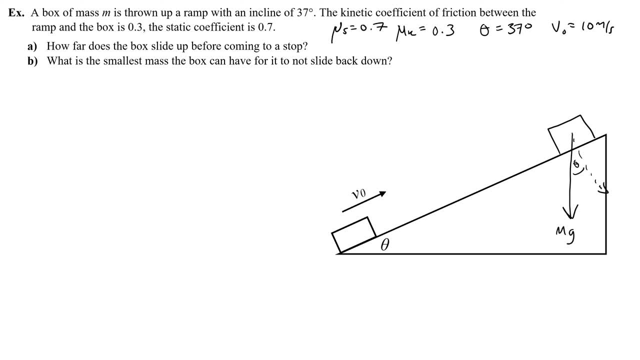 Okay, so it's still got. mg Theta goes there. This is going to be mg cosine theta And this will be mg sine theta. Then there's going to be a normal force up, And the question is, once the box has gone up to its highest point. 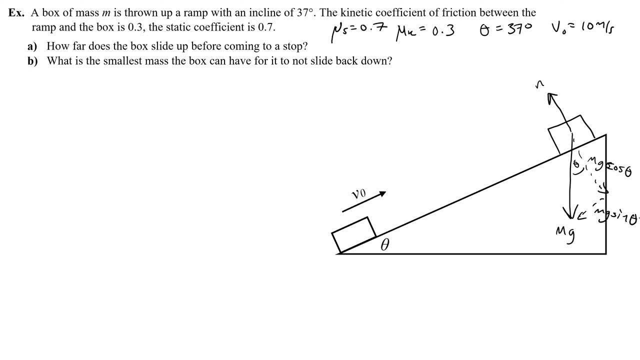 what direction should I draw friction in? Remember, as the box went up the ramp with that velocity, the friction force acted down the ramp, helping gravity to slow the box. However, at the very very top, suddenly, the box has stopped. 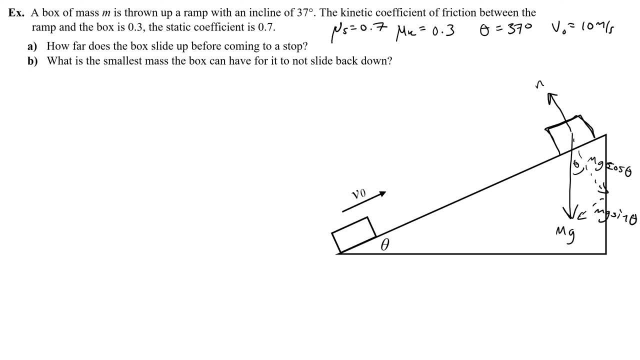 and it isn't moving up the ramp. Now it's stopped And this component of weight, mg sine theta, is trying to pull the box down, And against the box's motion, against that force, is our static friction. Now the idea here is that 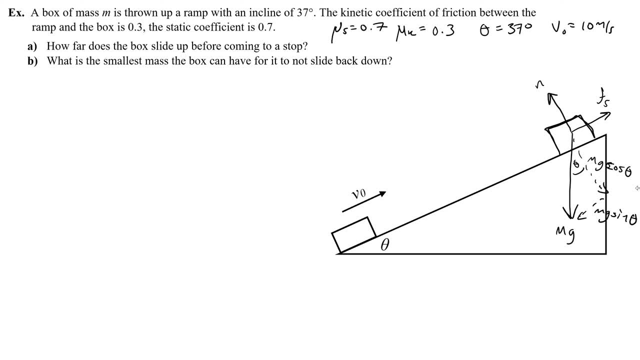 for one brief moment. the box and the ramp are going to be stuck together And it's going to be static And we're going to see whether or not the box has enough static friction to keep the box stuck at the top of the hill. 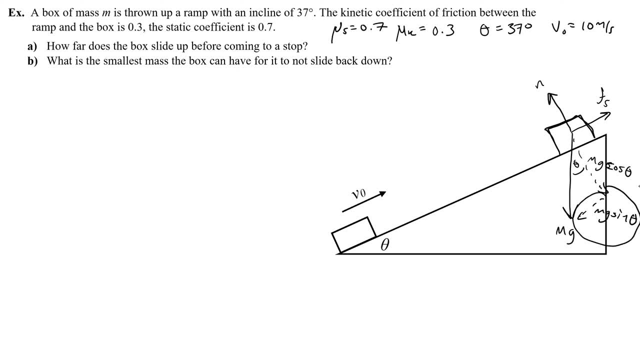 or if the weight force ends up being bigger than that static friction and it comes down. So what we're talking about at the top is a question of S max And we're trying to think about the situation for when S max is equal to mg sine theta. 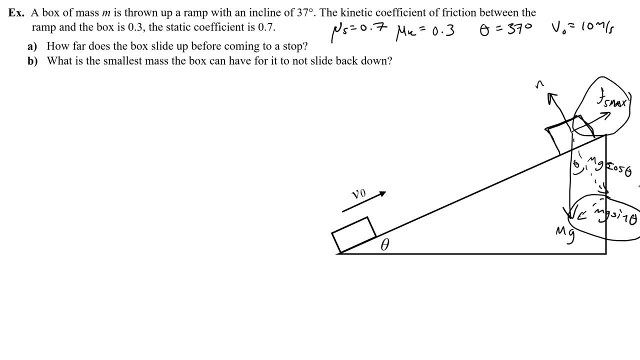 Okay, so at the top, if F max is equal to mg sine theta, then that lets us know the minimum maximum static friction that we need to have in order for the box to stop. If we have more static friction than mg sine theta. 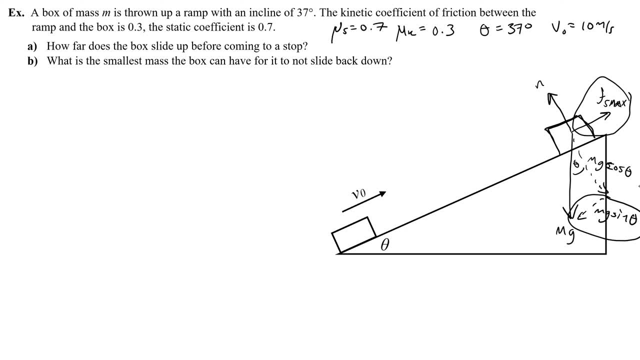 then that's great. it's not going to go down the ramp. So let's deal with this hypothetical smallest minimum situation Where again we're saying F max is equal to mg sine theta. Well, is there a way for us to compare? 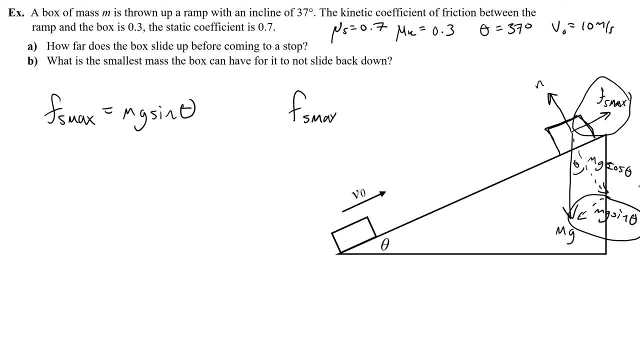 mg sine theta to F max. There is because we know that the maximum static friction is going to be equal to mu s, the static coefficient of friction times the normal force, And in this problem the normal force is equal to mg cosine theta. 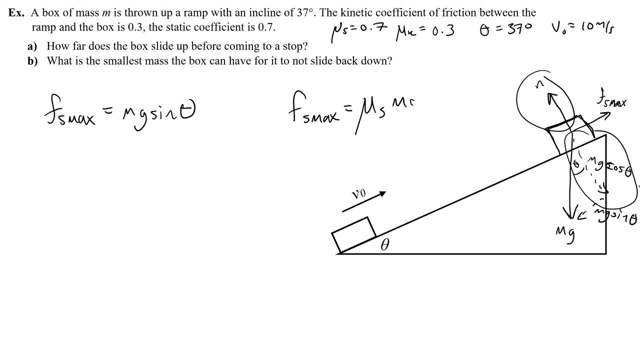 So really I should write mu s mg cosine theta. Well, wait a minute. That's super interesting, because now I can set these two equations equal to each other. Mu s mg cosine theta equals mg sine theta, And. 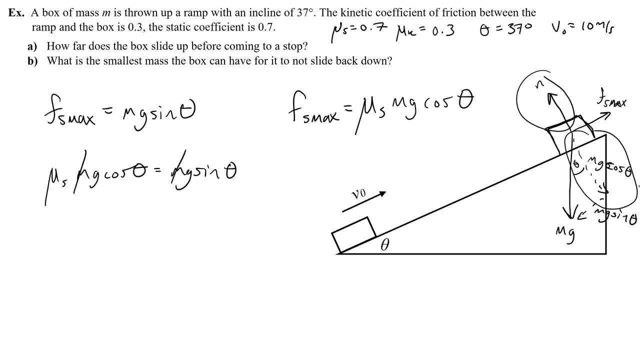 Wait a minute. M cancels out. So what's the smallest mass? Uh, That's kind of weird, right, Because the mass doesn't matter. So I guess the question becomes: does this box slide back down or not? 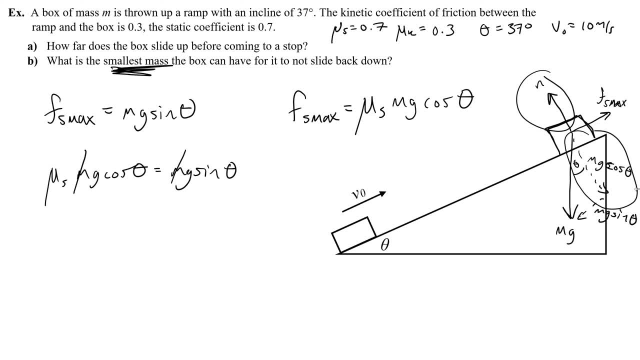 How do we figure it out? Well, here's what we do. We first of all get rid of g, because there's also a g on each side, And we get this equation: mu s cosine theta equals sine theta. 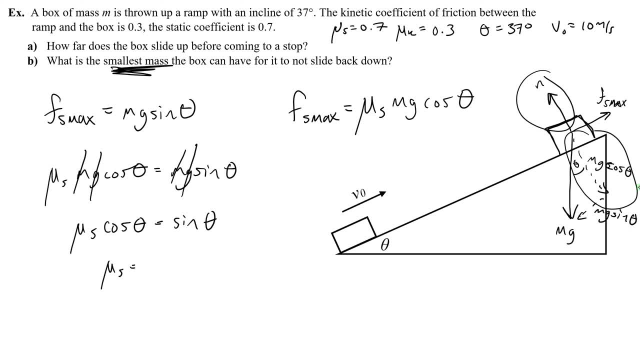 Then we're going to divide both sides by cosine theta, so we get mu s equals sine over cosine theta or tangent theta, And we get this really interesting equation. Now remember this is when the maximum static friction is equal to mg sine theta. 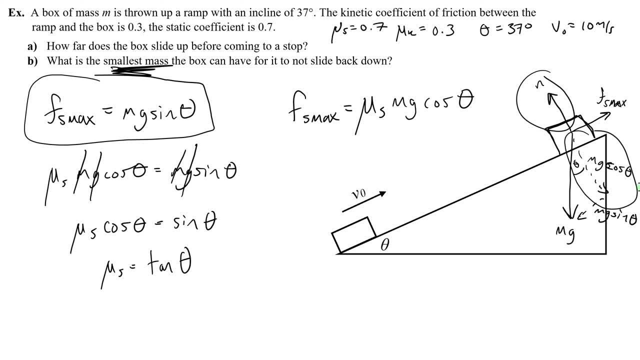 It's a hypothetical minimum. This maximum static friction could be more. It sort of depends on our problem. So what we need to do is we need to plug in our angle of 37 degrees and figure out what the coefficient of friction is going to be. 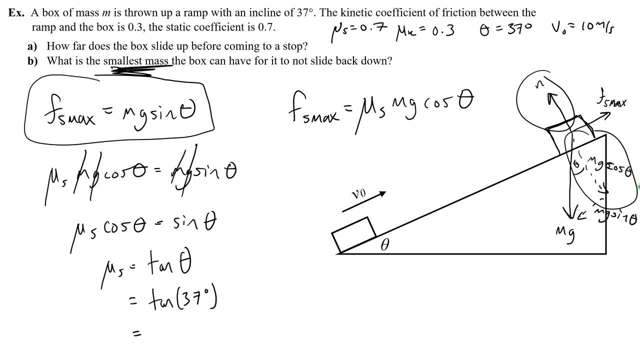 So tangent of 37 gives me 0.75.. So what we're saying is that, in order for there to be more static friction than mg sine theta, in order for the friction holding the box up to be at least equal to the weight, 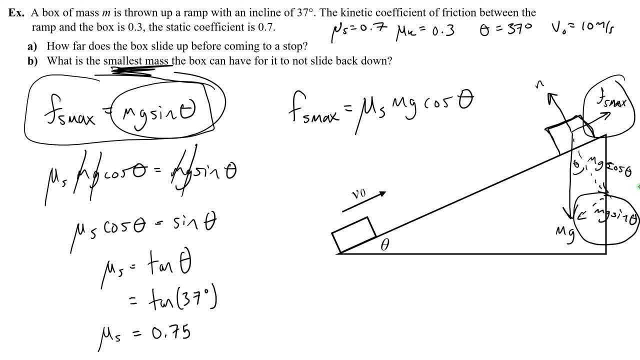 of the box trying to pull it down. we need to have a coefficient of static friction that is at least 0.75.. But guess what? Our static coefficient of friction is 0.7.. So that means that no matter how big 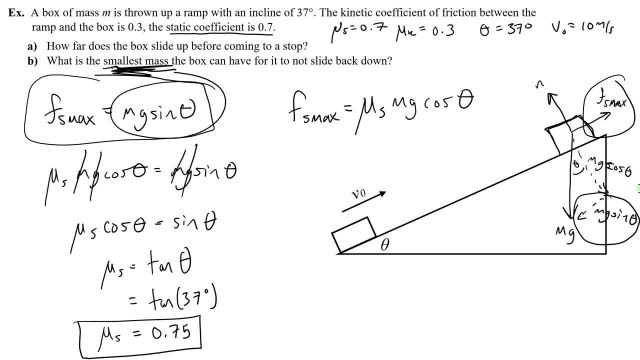 or how small the mass of the box is. it will never stay at rest at the top of the ramp. It could be 2 pounds, It could be 0.03 pounds, It could be 100 pounds, It doesn't matter. 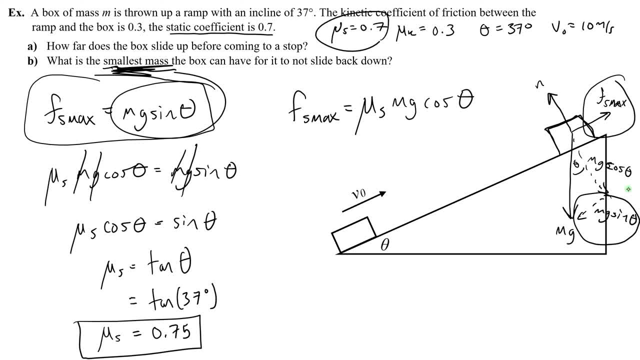 The box doesn't have a coefficient of static friction high enough for it to have a maximum static friction to balance mg sine theta. So we know that it comes back down And this is kind of a weirdly worded question, but you get the idea. 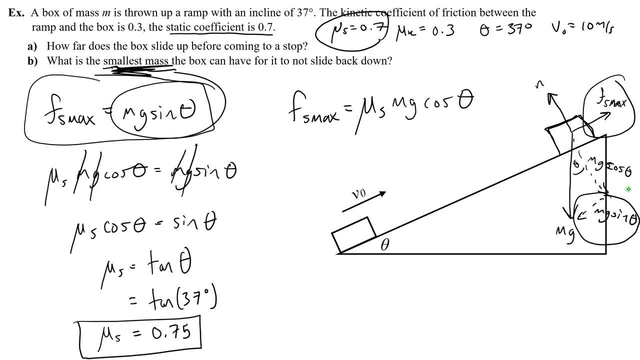 Okay, lots of thinking in this video and you did a great job. And remember mg sine theta and mg cosine theta. they're like the bread and butter. They are how we solve these kinds of problems and they are always going to be pretty difficult.